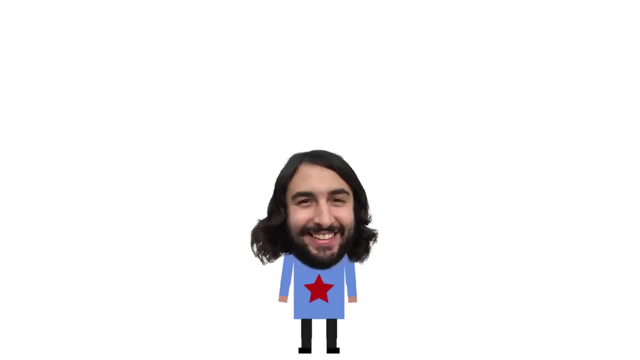 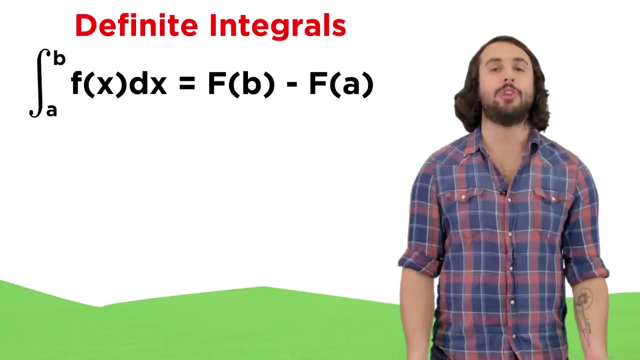 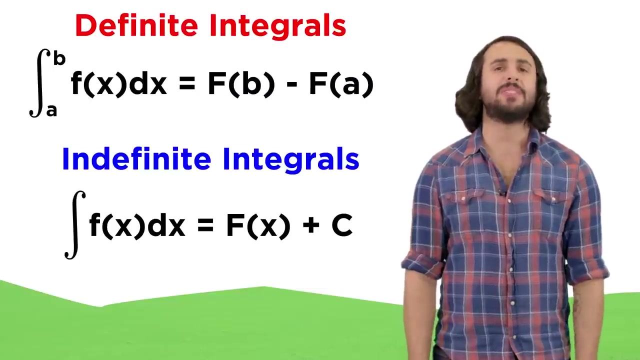 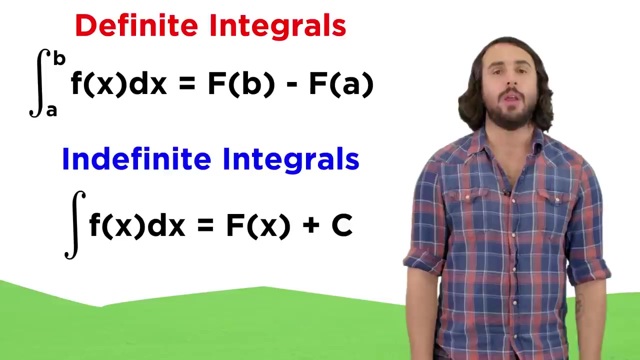 Professor Dave, here let's look at indefinite integrals. We now know how to evaluate definite integrals by evaluating antiderivatives over a specific interval, But sometimes we will be looking at integrals with no limits of integration listed. These are called indefinite integrals. 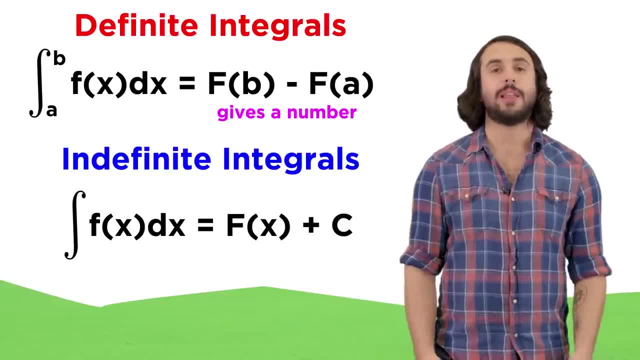 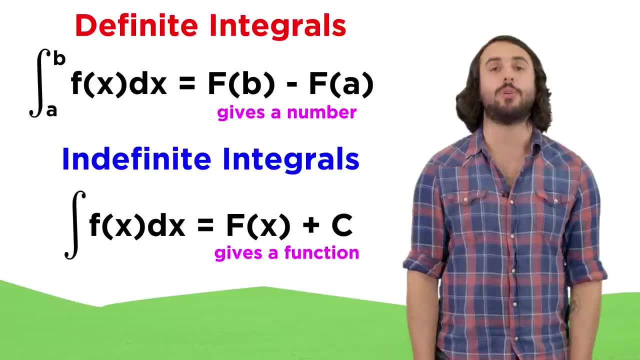 The main difference is that definite integrals are numbers like the area under a curve for a specific interval, but indefinite integrals, because there is no specified interval over which to evaluate, are actually functions or families of functions. This may seem totally different than what we have described integration to be thus far. 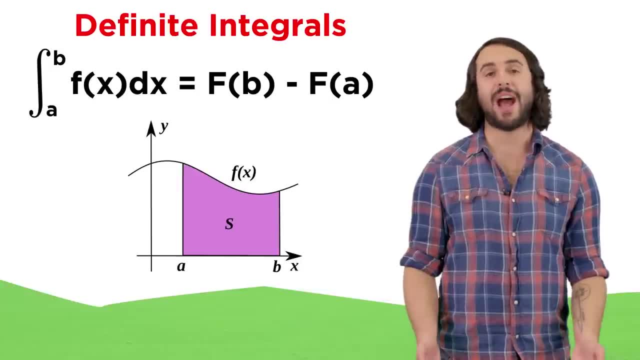 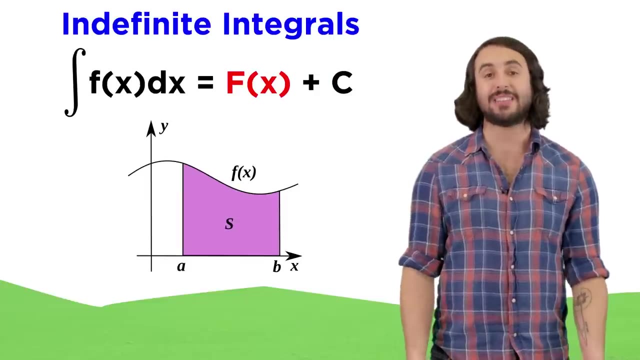 but if we think about it with definite integrals, we were simply evaluating the antiderivative over some arbitrary interval. If that interval can be literally anything and we can compute absolutely any definite integral from the antiderivative, then it follows that the antiderivative, the function itself, is the integral of the integrand in. 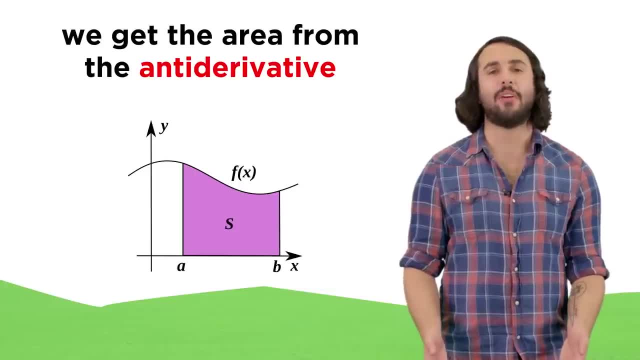 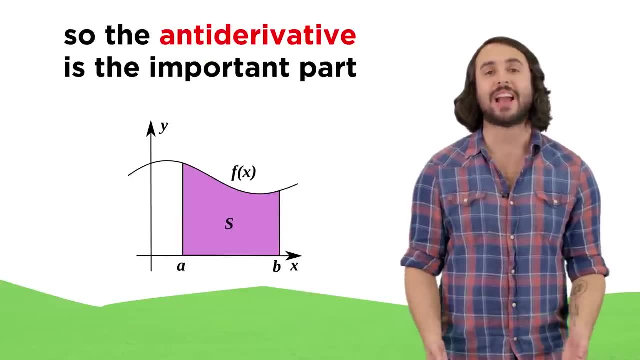 the truest sense. In short, we started off wanting areas under curves and found that we could get these from antiderivatives, so we're now just considering the antiderivatives themselves, Since indefinite integrals still involve the same process of finding the antiderivative. 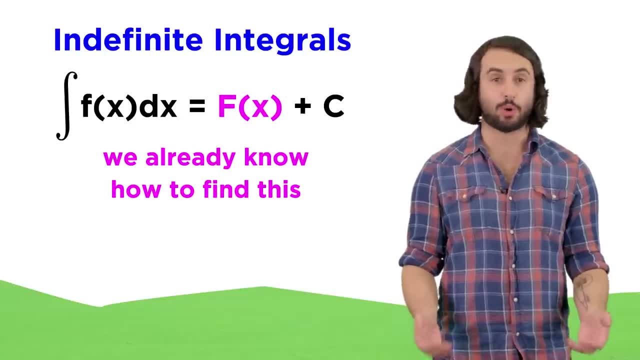 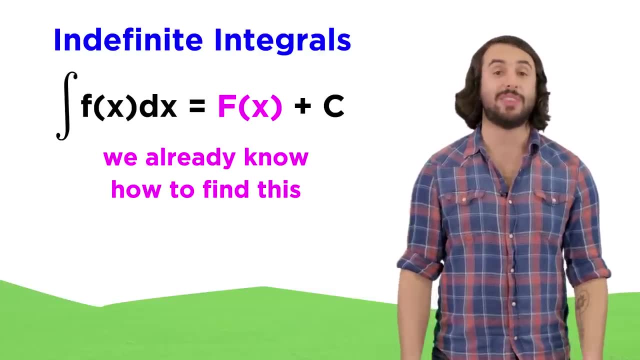 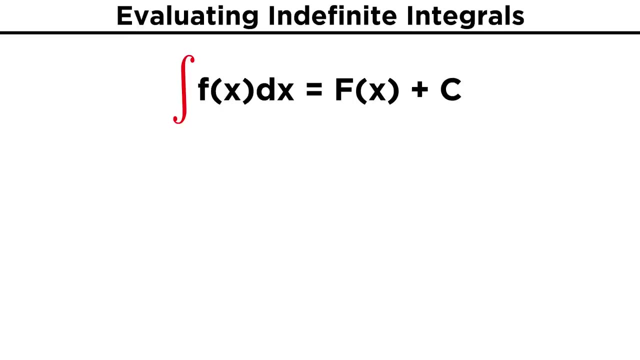 that evaluating definite integrals requires. it won't be that much different, but there are some important things to mention regarding indefinite integrals, so let's go over these now. As we said, indefinite integrals are ones with no limits of integration indicated. 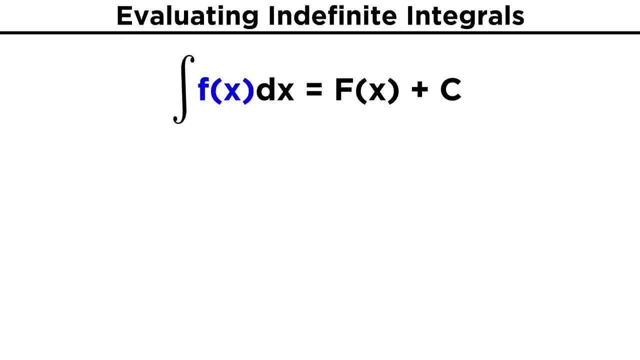 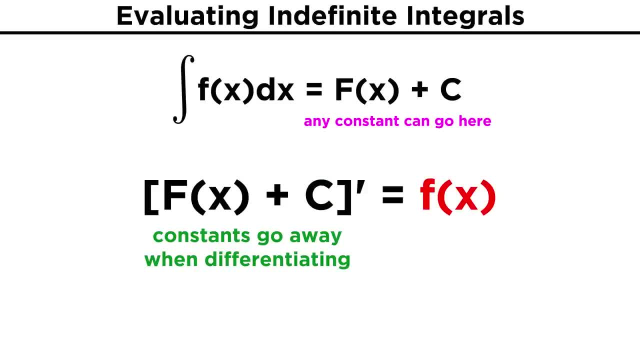 constant will simply go away, leaving us with F. So if we are integrating X squared, we will get X cubed over three, as we expected, but we also write plus C, meaning that any constant may be present. We didn't care about this when we were evaluating definite integrals, because, whatever this, 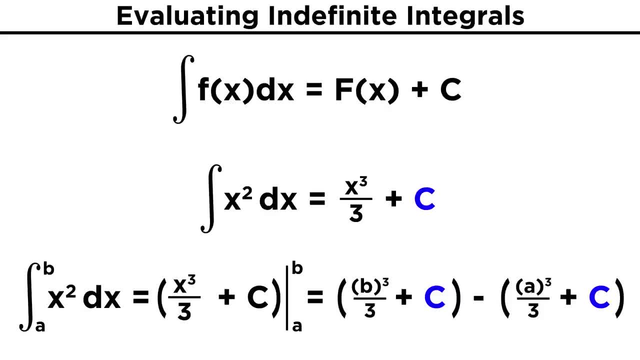 constant is, it would be present when evaluating at both the upper limit and lower limit, which means it will simply subtract and therefore not affect our result. But if we are looking at indefinite integrals, where we are simply writing a function, the 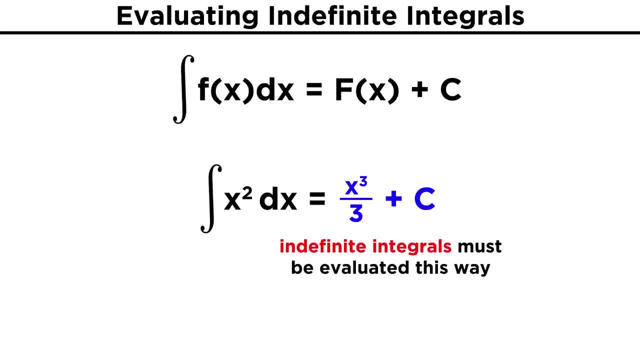 notion of this constant does indeed become relevant, and we must write it Just to clarify one more time, when we take the derivative of this antiderivative: X cubed over three becomes X squared, as expected, and the constant will go away, giving us the 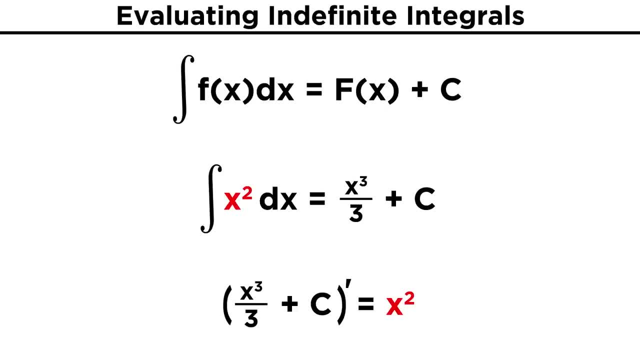 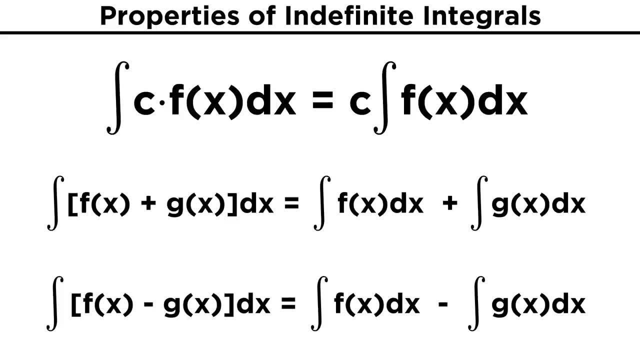 original function, So truly any constant could have been present. The properties of indefinite integrals will be precisely the same as those for definite integrals that we already went over. so just to review the integral of a constant times, some function will be equal to the constant times, the integral of the function. 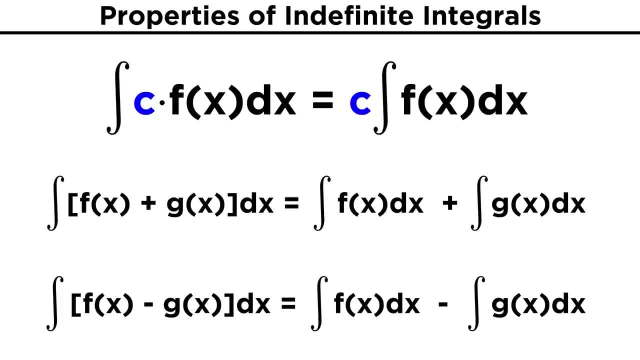 So make sure to remember that constants can be pulled out of integrals. Let's also recall that integrals are not always constant. Integrals of sums and differences can be split up into sums and differences of integrals, and this property will be very useful in certain circumstances. 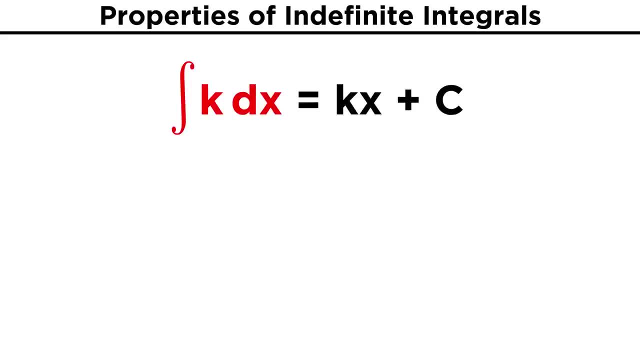 The integral of a constant with respect to some differential, like KDX, will always be the constant times. the variable, like KX here and then plus C for the reasons we mentioned earlier. And lastly, the property you will be using most frequently: the integral of X to the 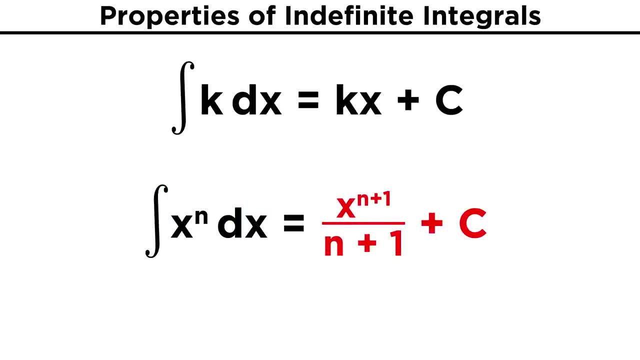 end, DX will be equal to X, to the N plus one over N plus one plus C. Remember, this is just the precise opposite process of taking a derivative, so that taking the derivative of the integral gives us back our original function, just as the fundamental theorem of calculus demands. 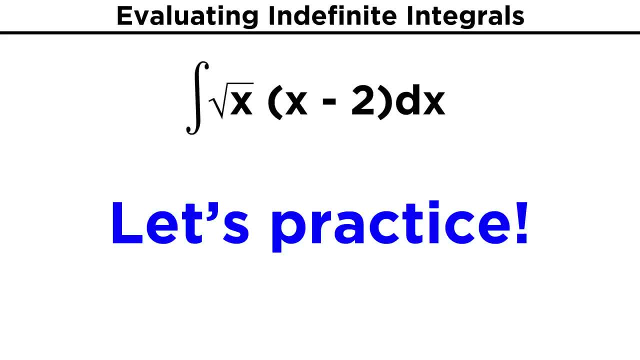 We have already practiced finding antiderivatives of polynomials when we used them to evaluate definite integrals. so just one or two practice examples. Let's try: root X times the quantity X minus two. To be clear, there is no product rule for integration, so this won't work the way. 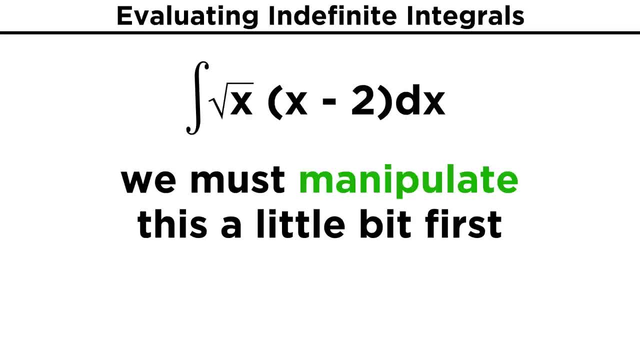 we are looking at it. We have to express this some other way. What if we change root X into X to the one half and then distribute that across this other term? That would give us X to the three halves minus two X to the one half. 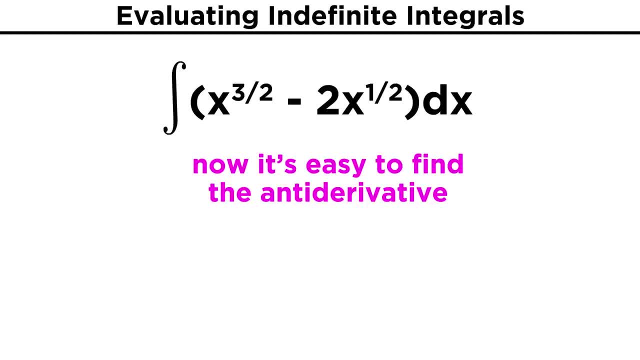 That's a little less appealing, but it doesn't matter, because now it is possible to find the antiderivative. so this is the way we have to go: Three halves plus one is five halves, so we get X to the five halves over five halves. 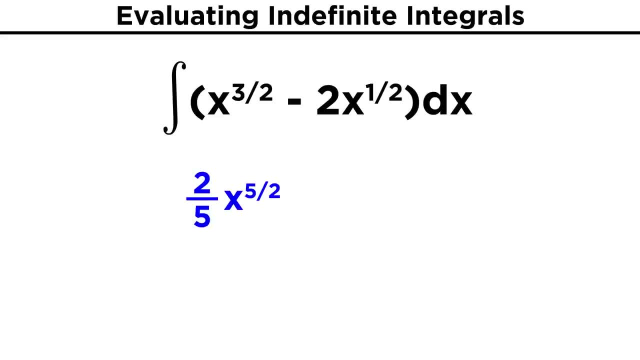 or two fifths X to the five halves. One half plus one is three halves. so for this term we get minus two times X to the three halves over three halves, or two times two thirds over three halves, or two times two thirds over three halves. 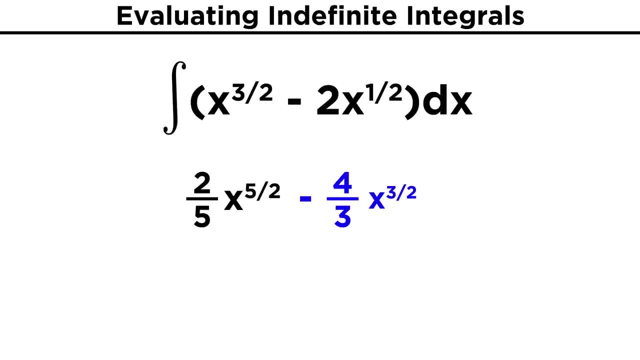 And lastly, as we discussed, if this were a definite integral, we could just evaluate this antiderivative over the limits of integration, in which case we don't have to worry about a constant, because any constant would disappear during the subtraction. 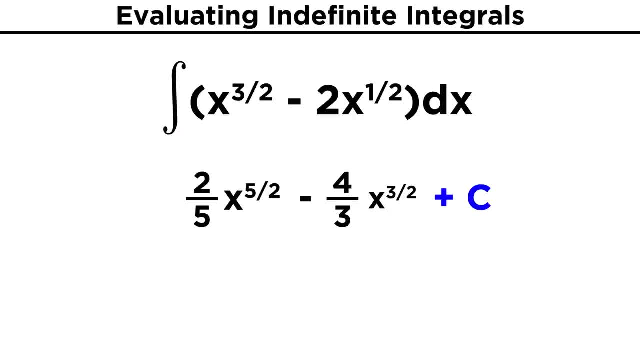 But as this is an indefinite integral, we do indeed have to write plus C at the end of this, because any constant can be here And this expression would be valid. How about another one? One over E to the negative X, plus one over three X. 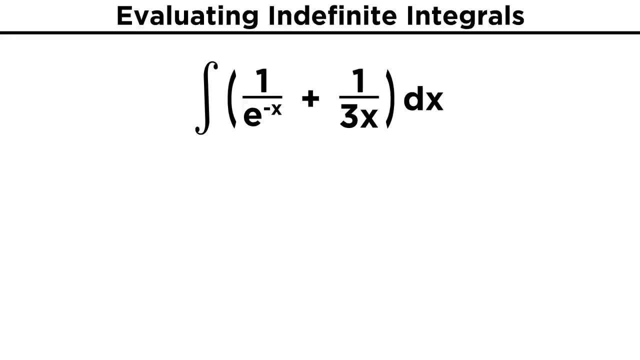 At first glance this seems complicated, but it's actually quite straightforward. First, since this is the integral of a sum, let's break it up into a sum of integrals to make things easier. Then, looking at the first one, if E is being raised to a negative exponent and is in the 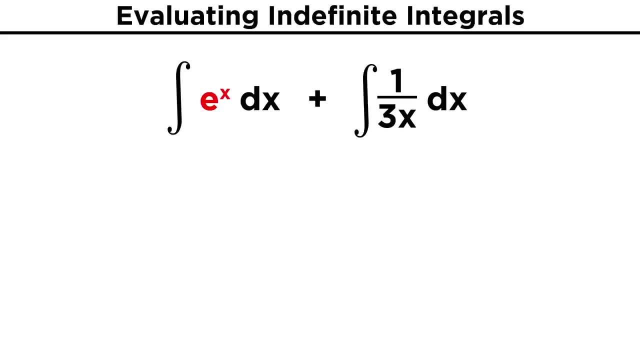 denominator. let's just bring it up to the denominator First. since this is the integral of a sum, let's break it up into a sum of integrals to make things easier. numerator and make the exponent positive. That will be e to the x. 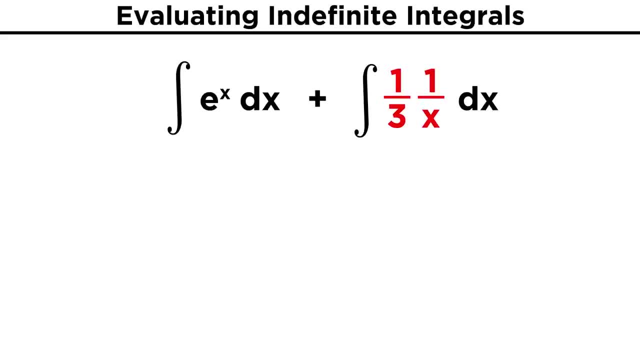 Then for this other term, this is the same thing as one third times one over x. From here to integrate, we just have to remember a couple things about the derivatives of special terms. When we looked at the derivatives of logarithmic and exponential functions, we learned the: 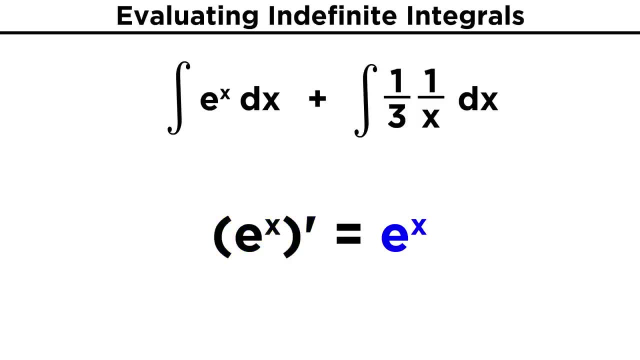 incredible fact that the derivative of e to the x is e to the x. It is the only function that does not change upon differentiation. But that means that if the derivative of e to the x is e to the x, then the integral of e to the x is also e to the x. 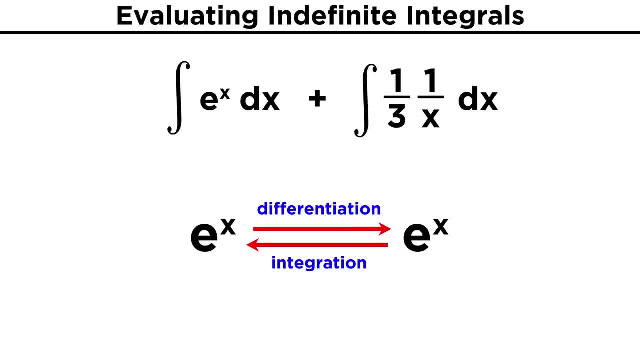 Whether we are going up or down on the ladder, e to the x doesn't change. So when finding this antiderivative, we can leave e to the x as it is. Then, for this other one, we must recall that the derivative of the natural log of x is: 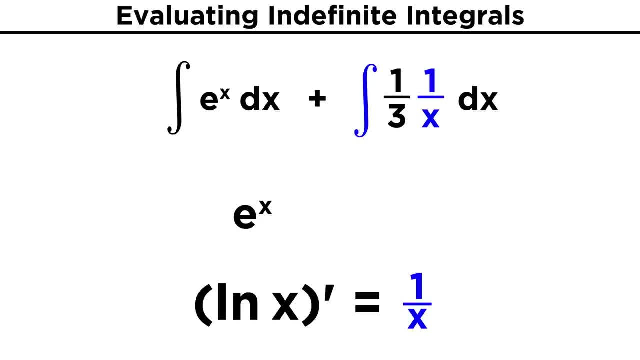 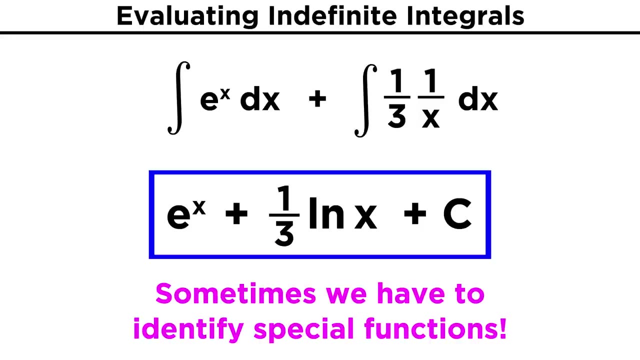 one over x. That also means that the antiderivative of one over x is the natural log of x. so this integral will be one third ln x. And lastly we add the constant c at the end. So sometimes we will have to identify special terms like these when integrating. 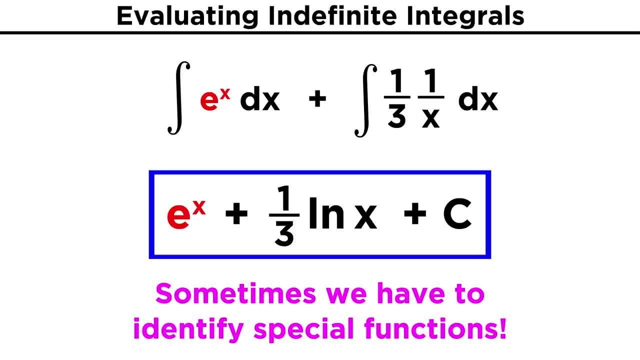 That e to the x remains e to the x is easy to remember. That one over x becomes natural log of x isn't so obvious as x to the negative one seems like it would follow the regular rule we use for any other exponent, but it is indeed the.